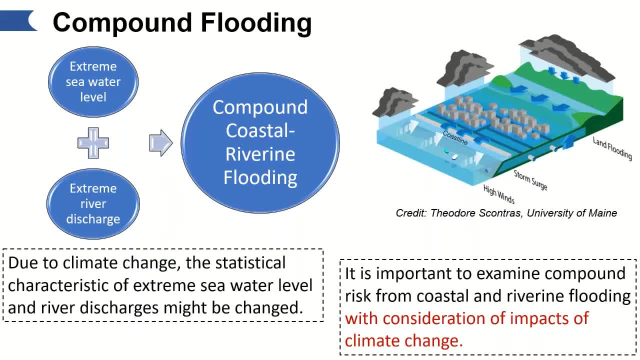 has increased over the past century at many coastal cities And this can be associated with the climate change. So it is important to examine the compound risk from coastal and river on flooding, with considering the impact of climate change. Slide 7, Slide 8: Sea level rise. 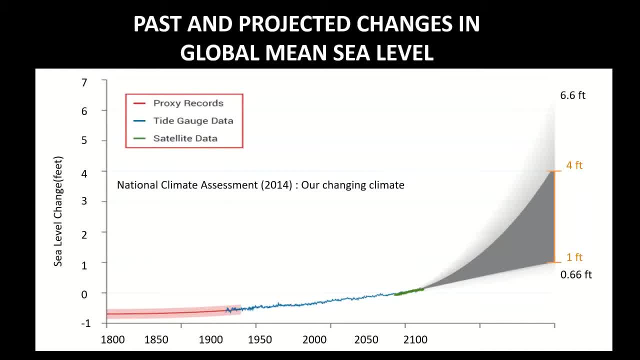 may be deemed as the most important impact of climate change in coastal regions. Here you can see the National Climate Assessment Sea Level Rise projection. What we can see here is that the global mean sea level has been increasing over the past decade And the rate of it is anticipated to accelerate over the 21st century. 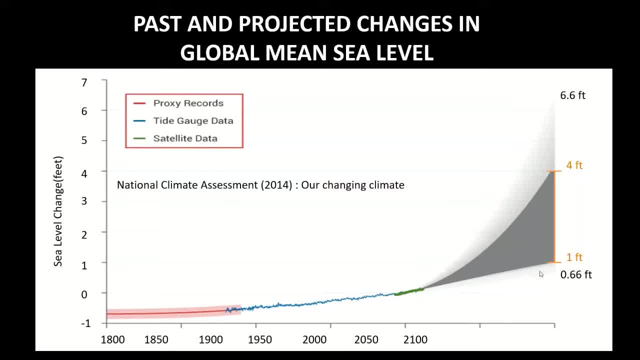 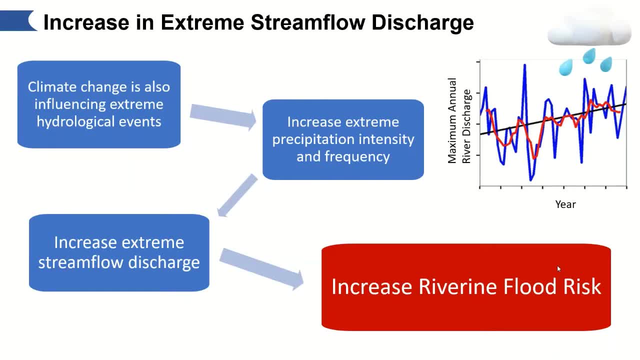 Slide 9 And also we can see that there is a great uncertainty in the future projection of sea level rise. climate change is also influencing extreme hydrological events, such as changes in extreme heavy precipitation intensity and frequency, which subsequently may lead to increase in extreme stream flow discharge, and these changes have an immediate impact on increased riverine flooding. 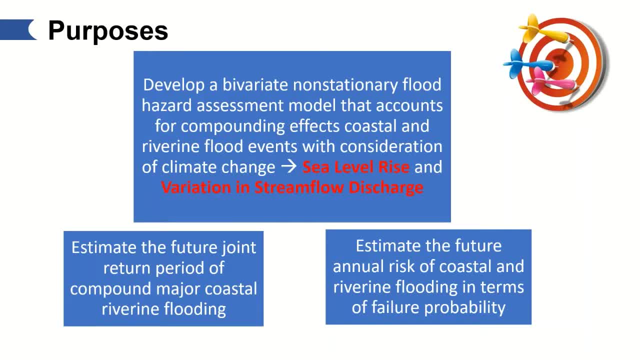 risk. so, with this information in mind, the main purpose of our study is to develop a bivariate non-stationary flood hazard assessment model that account for compounding effect of coastal and riverine flood events, with consideration of climate change, including sea level rise, and also. 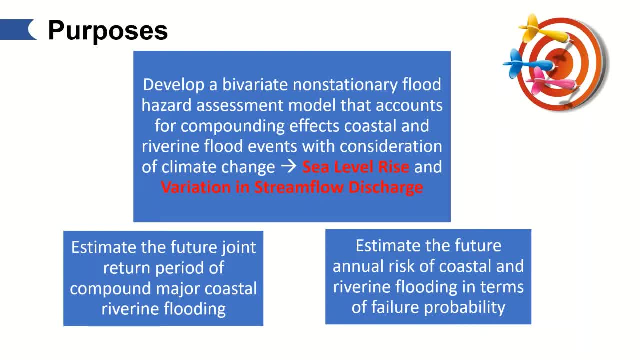 variation in the stream flow discharge and then to use this methodology to estimate the future joint return period of compound major coastal riverine flooding and also estimate the future annual risk of coastal and riverine flooding in terms of failure probability. and since we are interested in estimation of flooding hazard, we 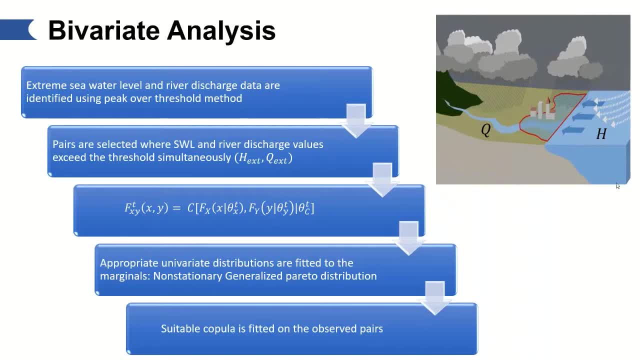 need to apply the bivariate model just to pairs of high values to prevent representation of extreme values with bias. so we use a pickover threshold method to identify extreme sea water level and river discharge risk, and then we use the bivariate model to estimate the future annual risk of coastal 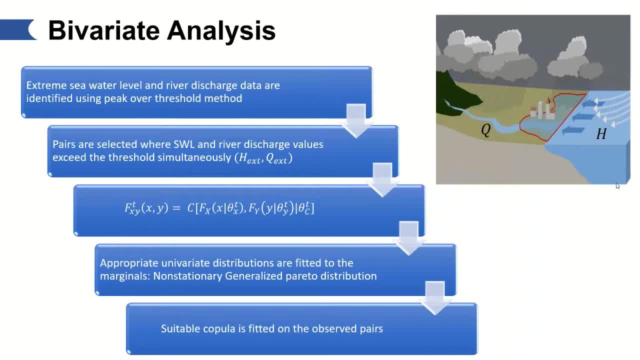 and river discharge data, and the basic idea behind this approach is to choose a threshold and to study the statistical properties of all exceedances over threshold for a given period of time, and it can be assumed that the exceedances above threshold follow a general generalized part of distribution, or simply gpd, and then we select the pairs when a sea water level and river 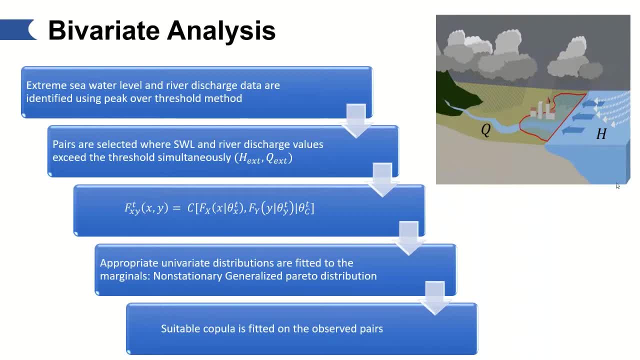 discharge value exceed the threshold, simultaneously to finally have the pairs of extreme sea water level and river discharge, and then these pairs of data should be fitted to the bivariate model. several parametric and non-parametric methods can be used for bivariate analysis, and we decided to use coppola methods, since using this method. 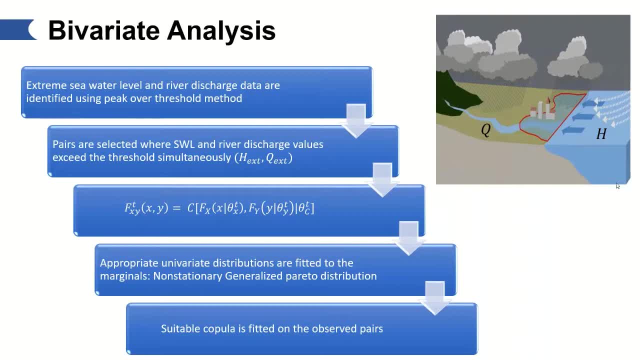 the marginal distributions can be selected without any limitation, and so for random variable x and y there is a unique coppola that describes the dependence structure between the random variables with marginal distribution of fx and fy. so we need to know the marginal distributions of the random variables and also their joint distribution, using coppola and, in general, the 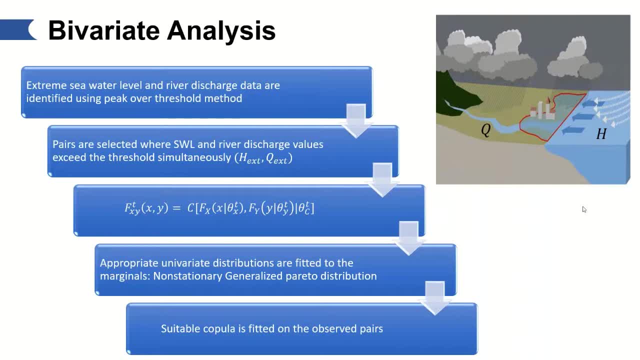 procedure is first to fit the best when you vary a distribution to the marginals, and then, since we use pickover threshold method to identify extreme pairs, a non-stationary gpd is used as a marginal distribution and then the best coppola is selected among 25 different coppolas based on: 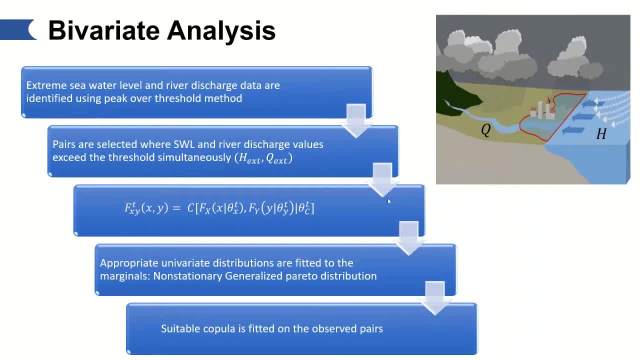 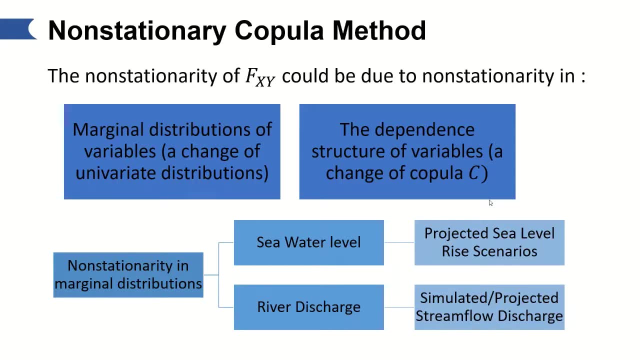 the bayesian information criteria, um. as i mentioned, our main goal is to incorporate the effect of climate change in our bivariate blood hazard assessment. so either the marginal distributions or the dependence structure between variables, or both can be non-stationary. uh, in this study we consider the non-stationary effects of climate change in 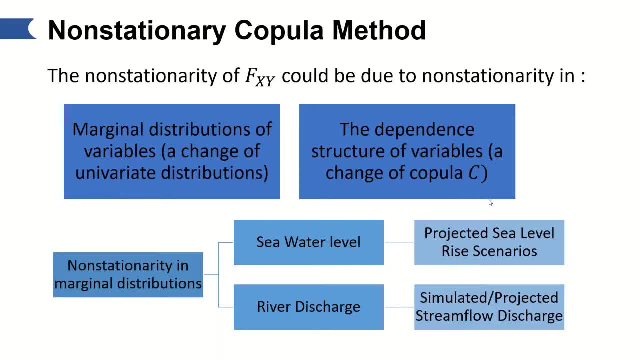 marginal distribution of sea water level and river discharge, and in order to do this, we use projected sea level rise scenarios and also projected streamflow discharge under different climate models. and so one more point before we move on to the next slide is that we have a very interesting 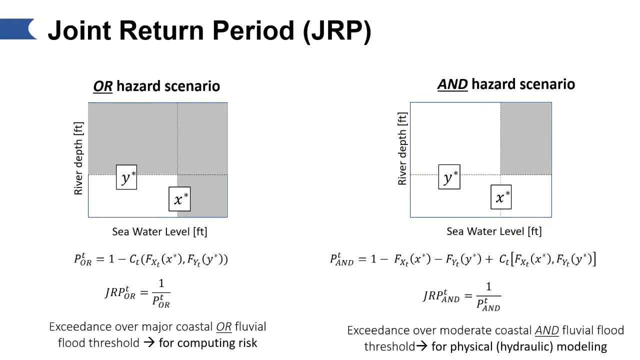 ity of the the bivariate analysis in in ripley charts. so this is a template. 10 here before i get to some results. unlike univariate analysis, joint written period is not unique in bivariate analysis and several consider exceedances above either coastal or river flood threshold, or both. The or scenario. 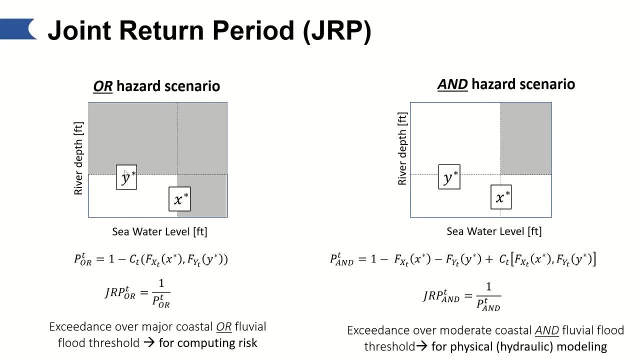 should be considered for computing risk, since either exceeding over coastal or river flood threshold, or both, is sufficient to produce flooding events And, as our scenario, consider the situation when both scenarios happen simultaneously. I mean that both river and coastal flood threshold are exceeded. This scenario should be considered for hydraulic modeling, which 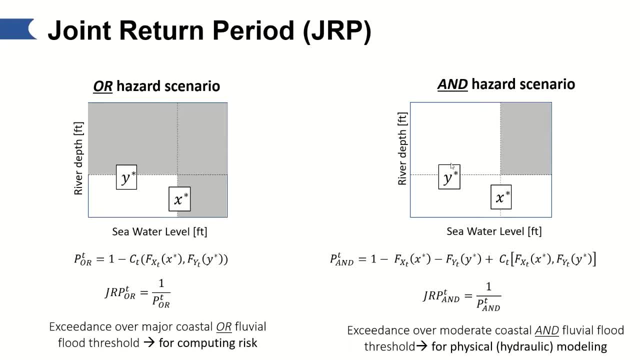 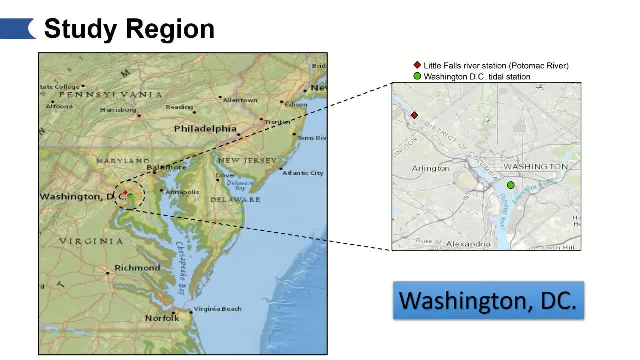 we need to know the probability of simultaneous occurrence of high sea water level and river discharge. We use the data from tidal and river station at the Potomac River estuary in Washington DC as a case study to demonstrate the application of our method. The green circle shows the location of Washington DC tidal station. 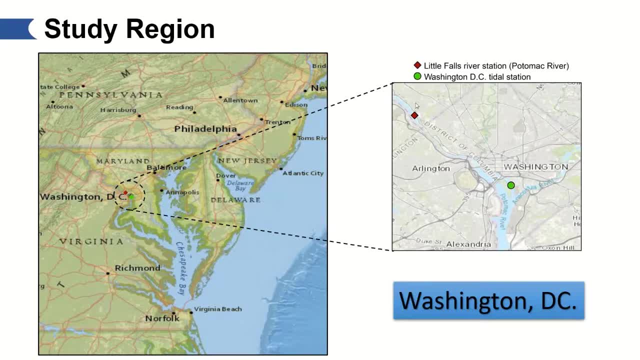 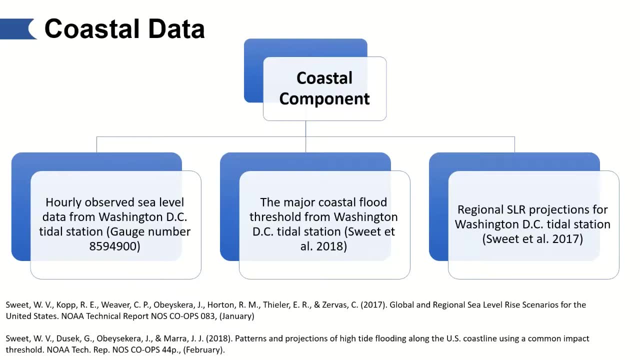 which is operated by NOAA, And the red one is Little Falls River Station at Potomac River, which is operated by USGS. For coastal component we need three sets of data: Hourly observed sea level data from Washington DC tidal station. also the major coastal flood threshold Since 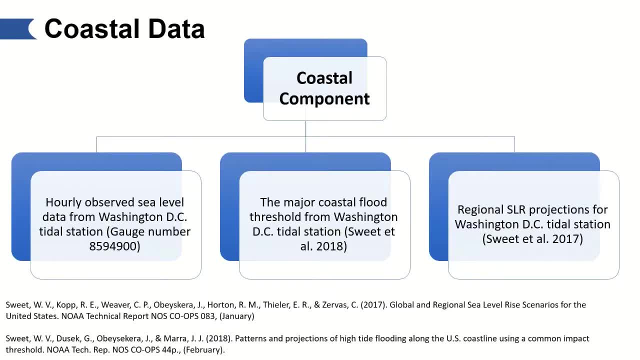 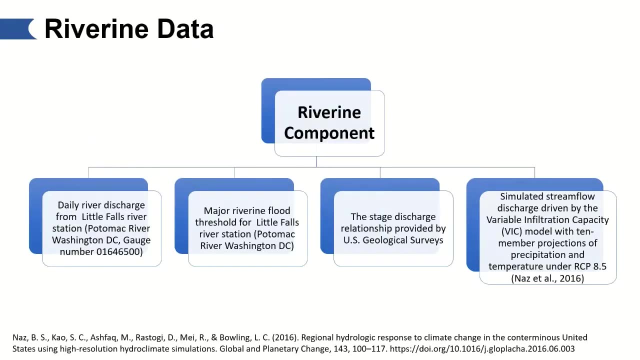 we are interested in characterization of major coastal river and flooding. this data was obtained from a report by SUIT, And also regional sea level rise projection scenarios, which was obtained by another report by SUIT. For river and component, we need four sets of data. First, daily river. 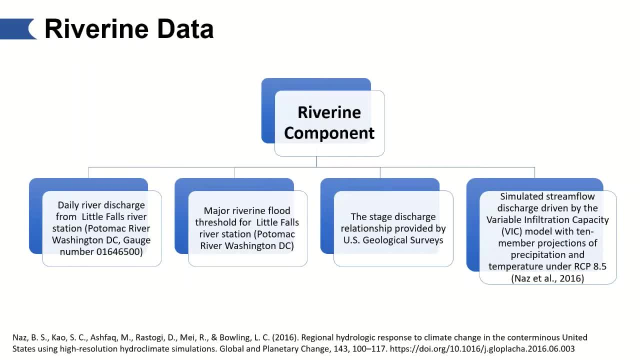 discharge from Little Falls River Station, also major river and flooding threshold, and also the sage discharge relationship for converting discharge values to depth, which all are obtained from USGS website. And finally, simulated streamflow discharge for incorporating non-stationarity in our model, which, for this study, we use: simulated streamflow discharge. 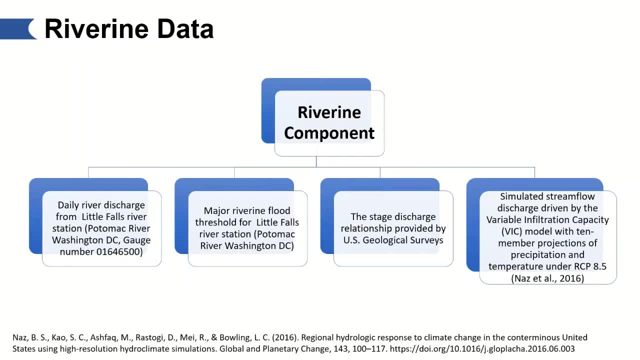 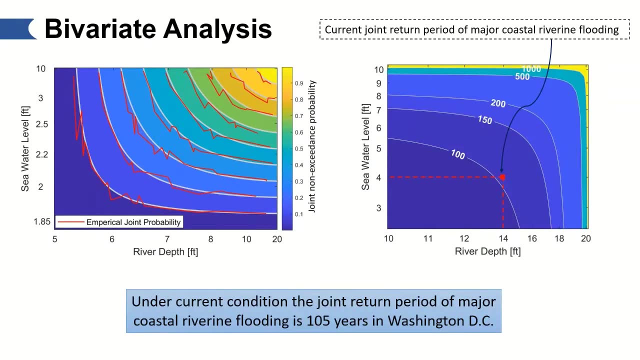 driven by the variable infiltration capacity, or simply weak model with 10-member projections of precipitation and temperature under RCP 8.5.. We used this data to explore the dependence between extreme sea water level and river depth in Washington DC. So after feeding the marginals to the GPD and selecting the 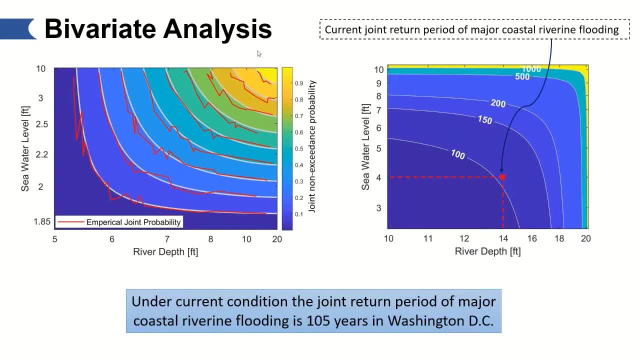 best cupola. we created the joint non-excident probability isoline, which you can see them in the left figure by gray lines, compared with the empirical joint non-excident probability isoline which here are shown by the red line. In the white figure you can see the current joint return period of simultaneous exceedance. 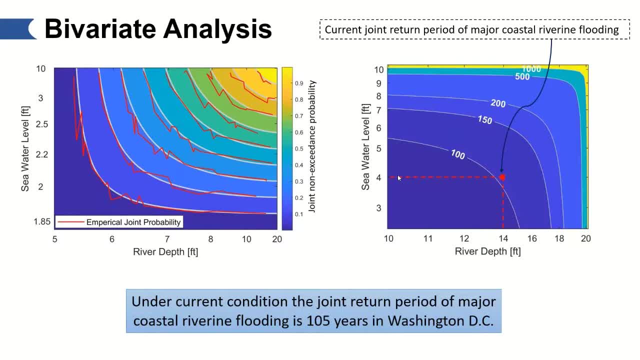 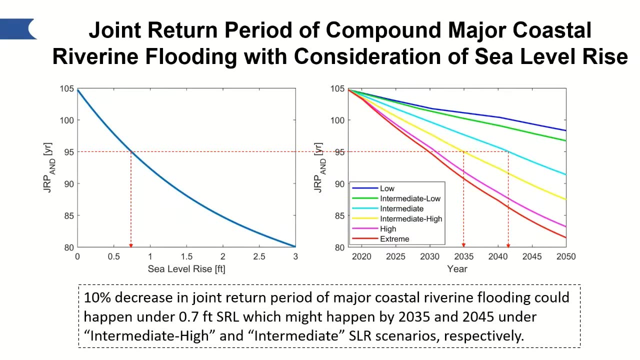 of different sea water level and river depth based on the end scenarios, And so you can see that the current joint return period of major coastal river and flooding is 105 years. However, as I discussed earlier, this value is not constant under climate change, So in 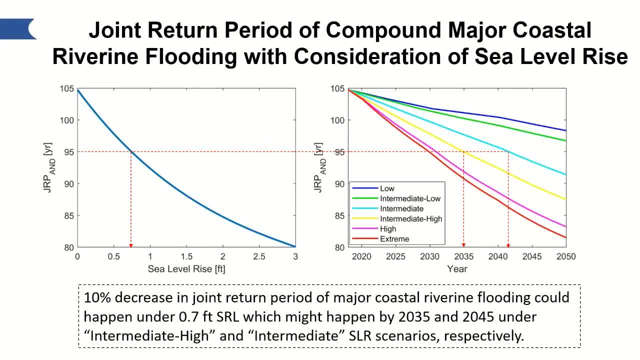 the first step, we estimate the joint return period of major coastal river and flooding Under different sea level rise values. You can see the result in the left figure. For example, we can see that 10% decrease in joint return period of major coastal river and flooding could happen under 0.7 feet sea. 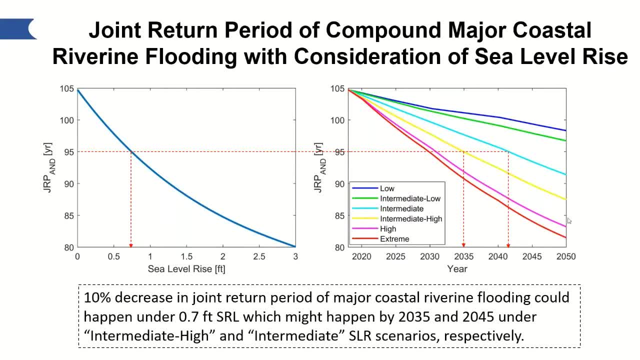 level rise. Then we use projected sea level rise scenarios to determine the time when indicated sea level rise are anticipated to occur. So we can see this 10% decrease in joint return period of major coastal river and flooding might happen by the year 2035 and 2045 under intermediate high and intermediate sea level. 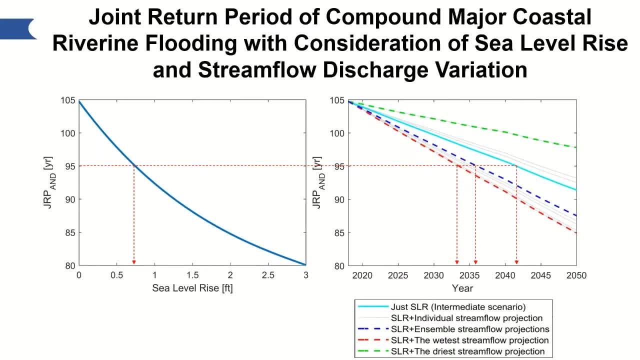 rise scenarios respectively. In the next step we also consider the effect of variation in extreme flow discharge and estimation of future joint return period of major coastal river and flooding, So we can see this 10% decrease in joint return period of major coastal river and flooding might. 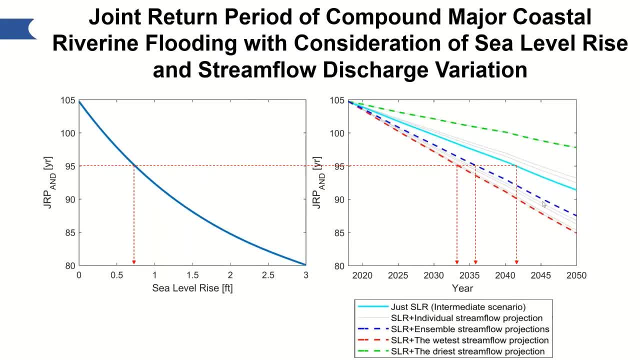 of major coastal riverine flooding. In the right figure you can see changes in the joint return period under just intermediate sea level rise scenario, which is shown in the right blue and intermediate sea level rise scenario with ensemble of stream flow prediction in dark blue And then the combination of intermediate sea level rise scenario and 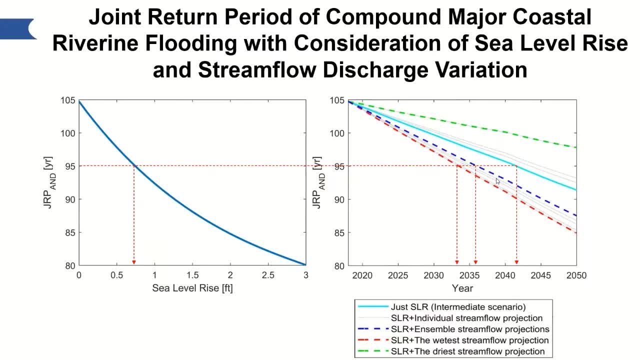 driest and wettest stream flow projections are also shown by green and red dashed line respectively. The point here is that the effect of sea level rise on changes in joint return period of major coastal riverine flooding is higher than impact of increasing the stream. 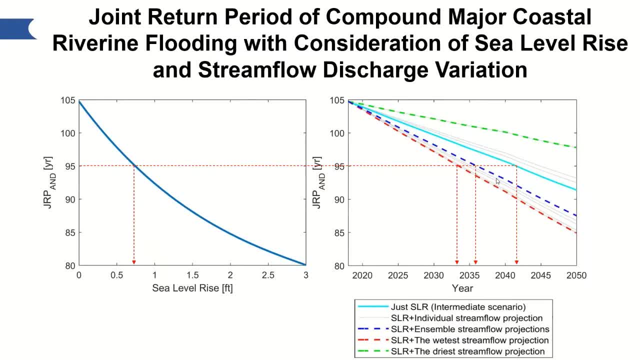 flow discharge 00.01.00. So, for example, by the mid-century we can see that there is almost 20% decrease in joint return period of major coastal riverine flooding, which almost 15% of that is due to sea level. 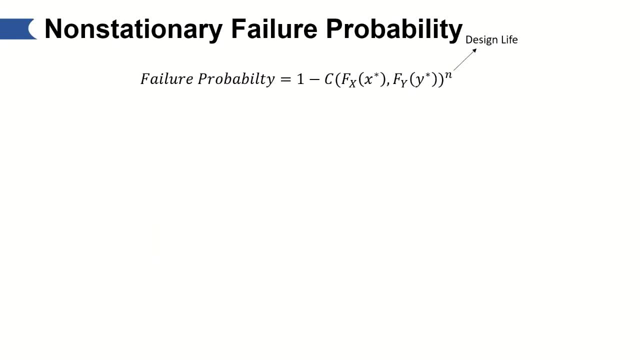 rise. Then we use the ore hazard scenario to estimate risks in terms of failure probability. Traditional stationary failure probability is 1 in 2.. In general, the first target in 2014 for univariate analysis- And then, using sea level rise scenario, we estimate the increase in failure probabilities. 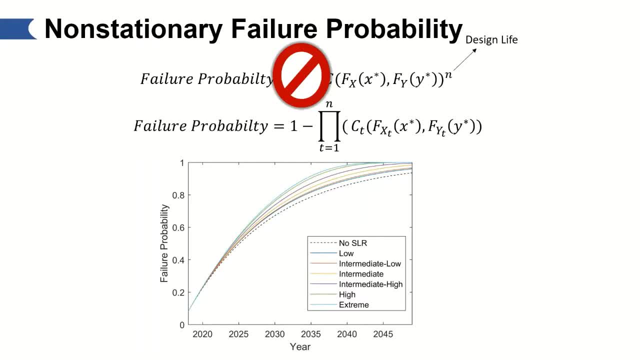 due to compound major coastal riverine flooding. major coastal river and flooding, And also failure probability under stationary condition is also presented by dashed black line for the sake of comparison. These results show the importance of considering sea level rise in estimation of failure probability and how. 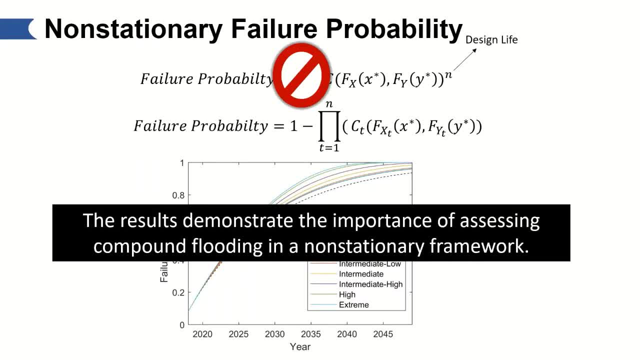 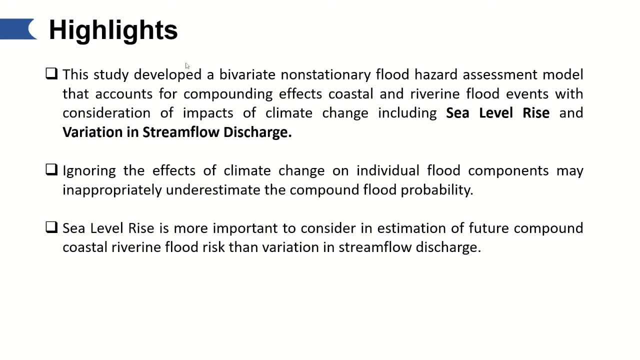 ignoring the effect of sea level rise leads to underestimation of future risk. So, in conclusion, this study developed a bivariate non-stationary flood hazard assessment that account for compounding effect of coastal and river and flooding events, with consideration of impact of climate change, including sea level rise and variation in stream flow. 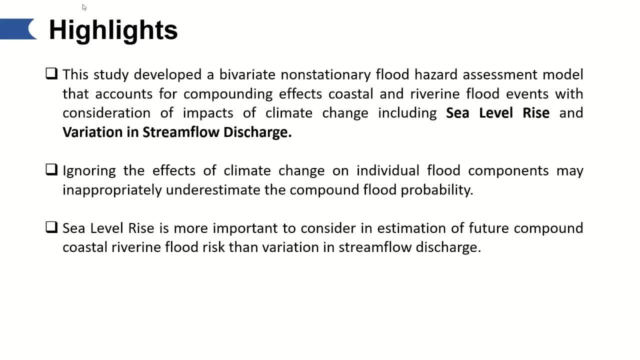 And then we found that ignoring the effect of climate change on individual flood component may lead to inappropriately underestimate the compound flood probability. And also we found that sea level rise is more important to consider in estimation of future compound flood risk compared to the variation in stream flow discharge. Thank, 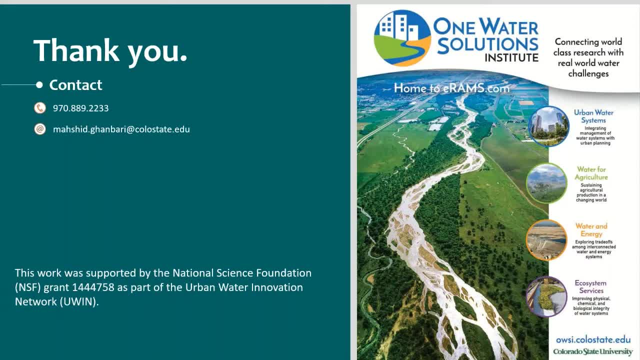 you. Thanks, Basheed. Well, I'll open it up for questions now so you can enter those into the chat queue or raise your hand and I'll turn your microphone on. Okay, Tim, it looks like you should be cleared. 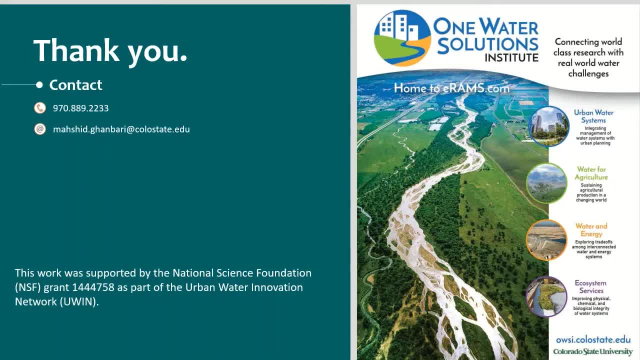 Yes, Hi, this is Tim Green. Thank you for the presentation. A couple of questions. One is so: when you look at sea level rise, you have a combination of larger scales and smaller scales and say storm surge and then the probability of storm surge combined. 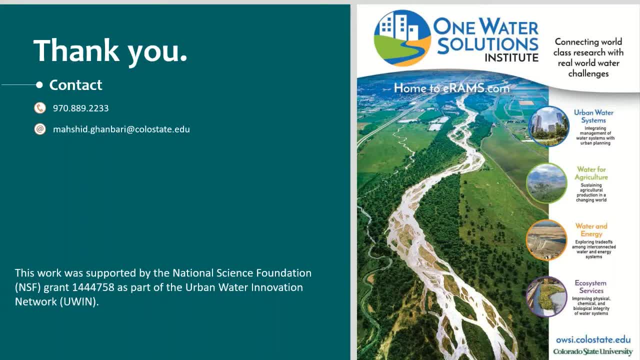 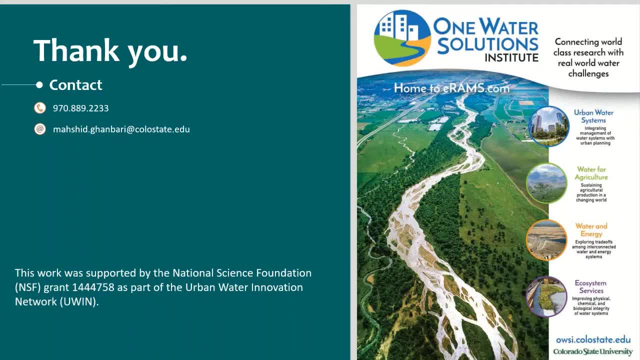 Basheed, I'm going to start with you, Basheed, I'm going to start with you, Basheed. So you have, say, those different components of sea level rise, And then with Chesapeake Bay, you have a very unique geometry. How would that compare with other parts of the world? 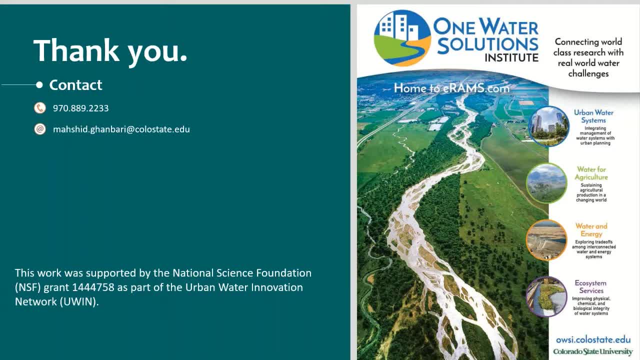 So this is a good question. We consider the all combination of sea water level- I mean the tide, the mean sea level and also the storm surge- together, And we didn't separate that because this is just a simple statistical analysis. Okay. 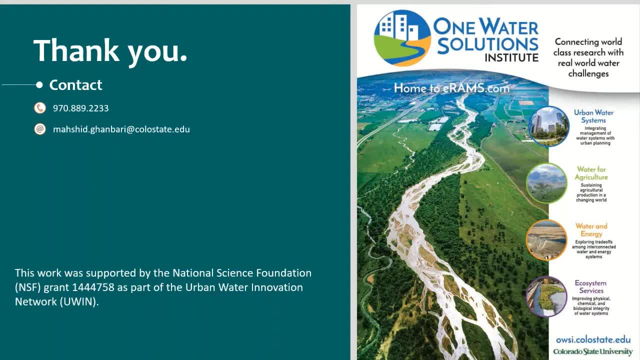 and we are not one to model this stuff, so we just use the combination of the sea water level. So our sea water level is the combination of the mean sea level, the tide and also a storm surge. We didn't separate that yet. 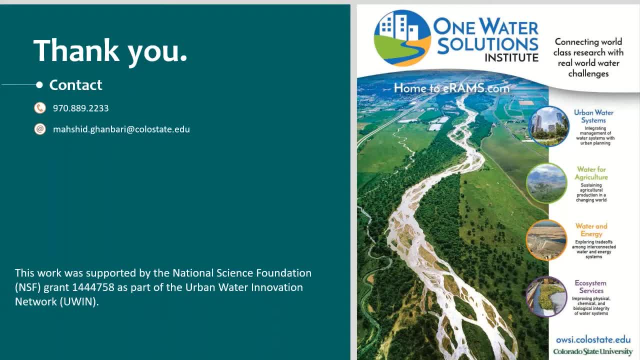 So do you have any sense of how it would compare to, say, a more open coastal area? I don't know. our plan is to use this statistical method for all the US and I don't know what would be the result for the other coasts, or I don't know. 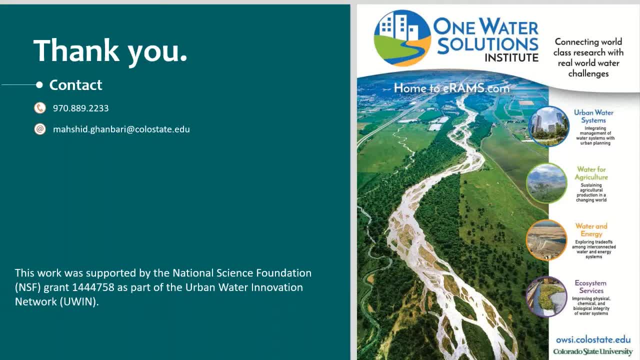 Okay, thank you, Sure, Okay. well, I haven't seen anything else come up and there's no other hands raised, So if there aren't any more questions at this time, I'll go ahead and get us transitioned to our next presenter. 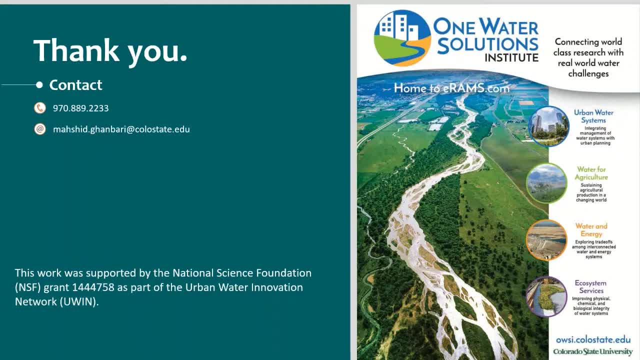 Thanks for your time, Mashied. Have a good day. Thank you, You too. 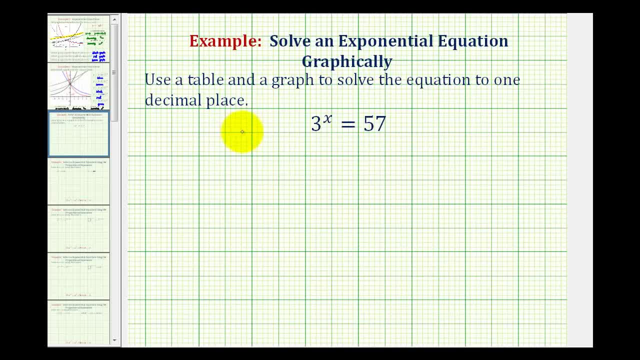 We want to use a table and a graph to solve the equation to one decimal place. We have: 3 raised to the power of x equals 57.. Notice how, if we could write 57 as 3 raised to some power, we could find the exact value of x. 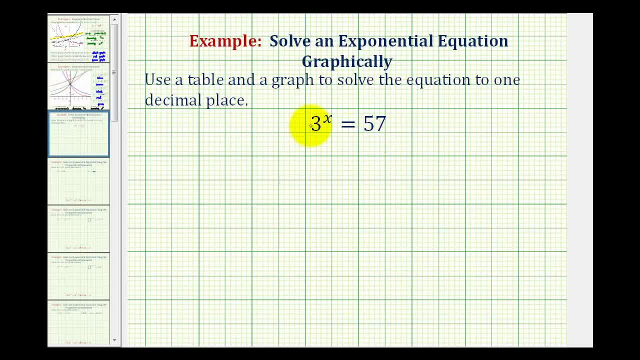 but since we can't, we're going to find an approximate solution. We will learn how to solve this type of problem using logarithms very soon, but for right now we're going to use technology. But we should recognize that 3 to the third would be equal to 27, and 3 to the fourth. 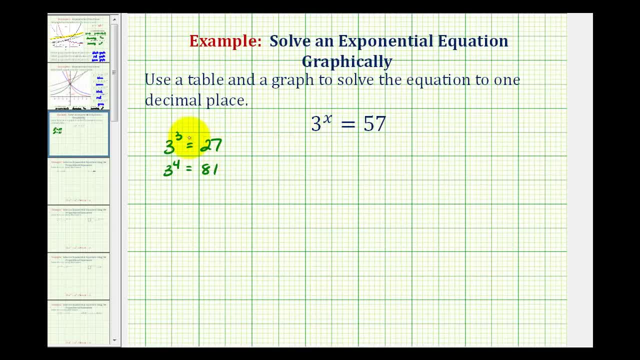 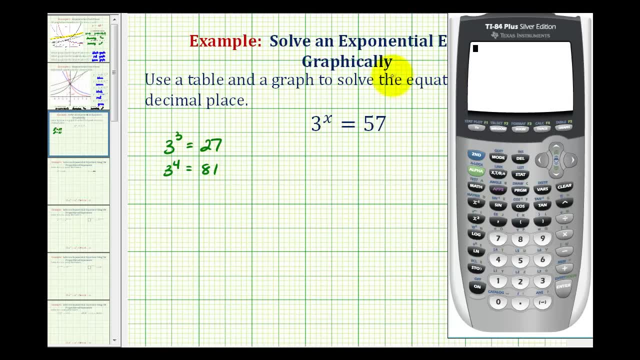 would be equal to 81, so the value of x would have to be somewhere between 3 and 4.. So let's get our graphing calculator out. The first thing we want to do is enter in y equals 3 to the power of x into the calculator. 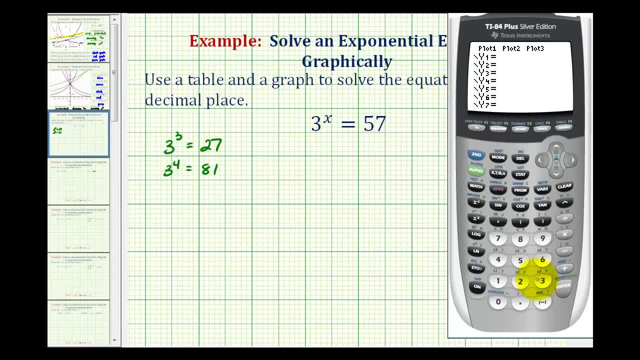 so we'll press y equals type in 3 raised to the power of x, and we'll start by solving this using a table. But before we go to our table, let's press second window for table set. Let's start the x value at 3..